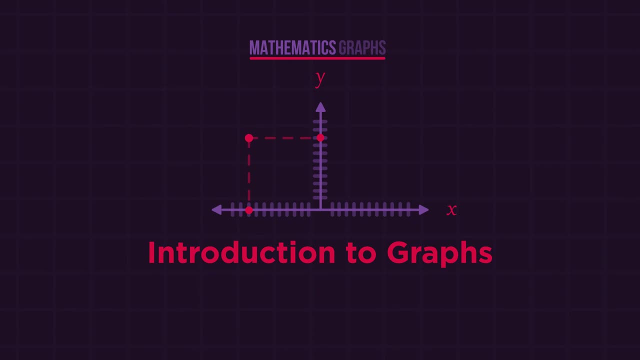 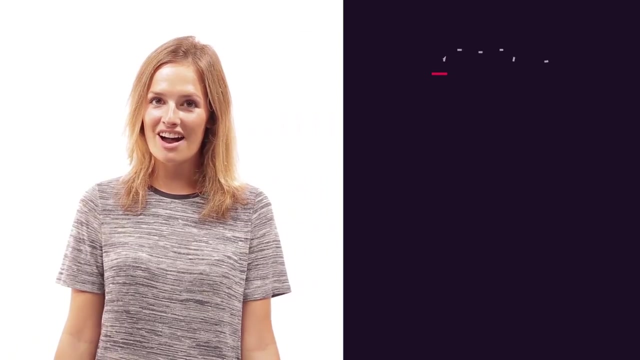 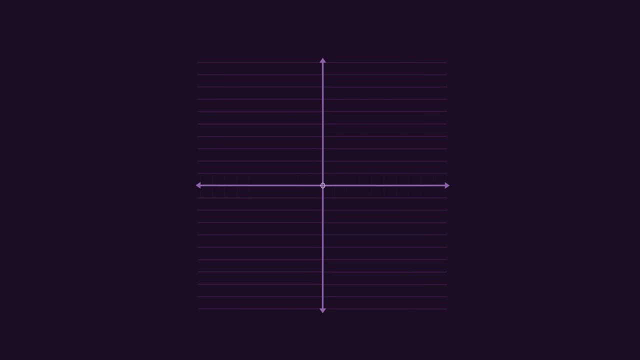 Hi, I'm Lucy and in this video we're going to learn all about the basics of graphs: What are axes, How do coordinates work And what are quadrants? Starting from the beginning, notice how the horizontal axis is called X and the vertical 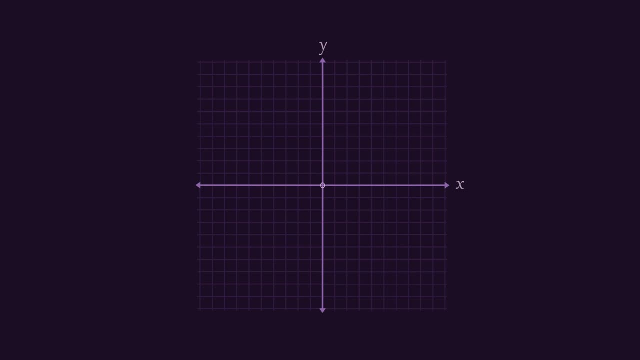 axis is called Y And they all start at zero, here in the middle, which is known as the origin, With the positive numbers going in these directions and the negative numbers going backwards and downwards. It's really important to remember that the X axis is the 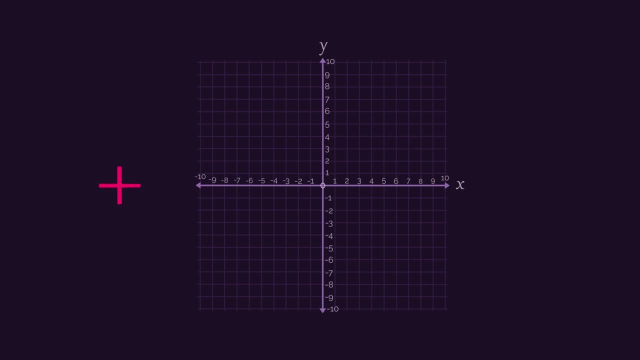 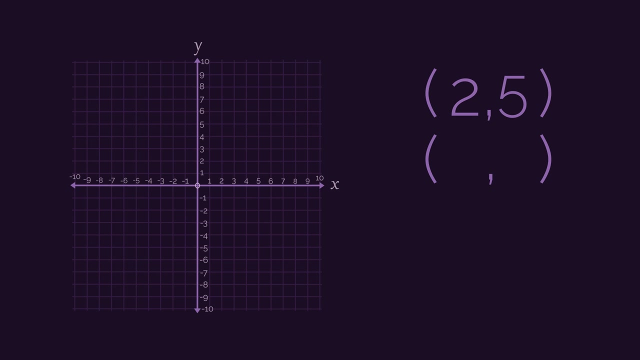 horizontal one. Just think: X is across, so X goes across. So now we know all about how the axes work. Let's make use of them. So coordinates are written as two numbers, separated by a comma and with brackets around. The first number is the X coordinate and the second number 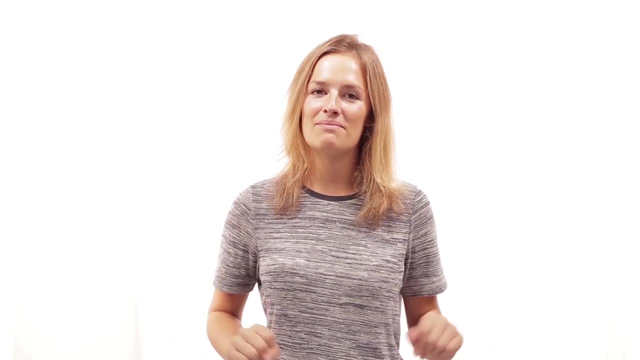 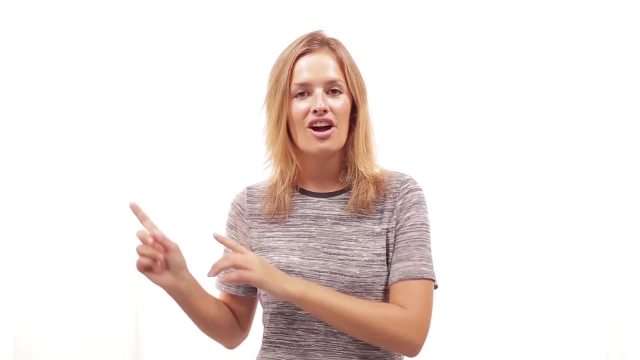 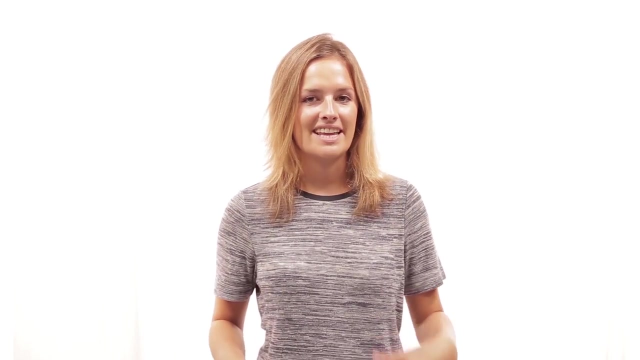 is the Y coordinate. This is easy to remember because the first numbers are long and the second one is up or down, because you have to go along the corridors before you can go up the stairs. Or you might just like to think about it alphabetically: X comes before Y. 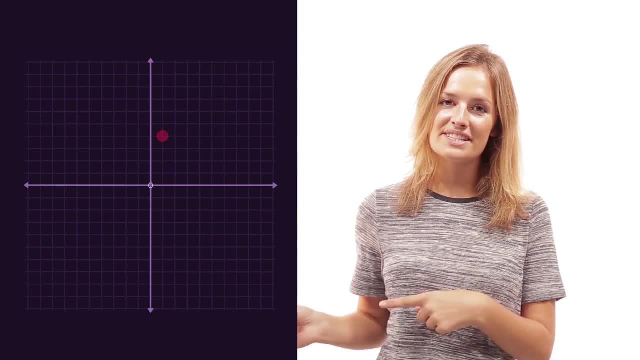 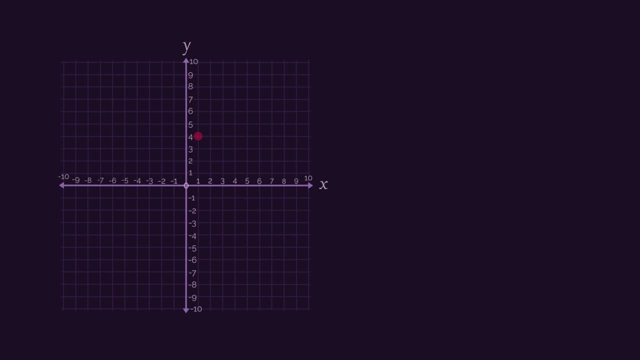 So what are the coordinates of this point? Pause the video, have a think and click play when you're ready. to check It is one four, because it is one along from the origin and four up. Where would negative four six go on the grid? Pause the video, have a think and click play when you're ready. 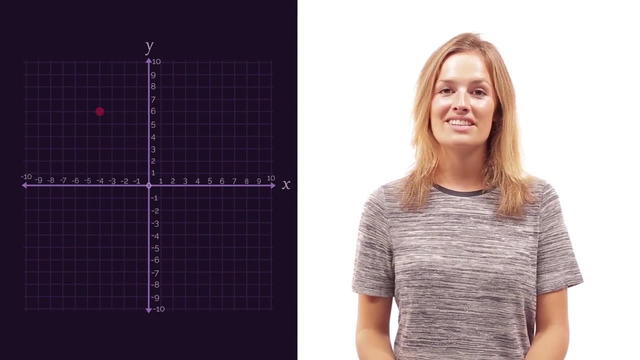 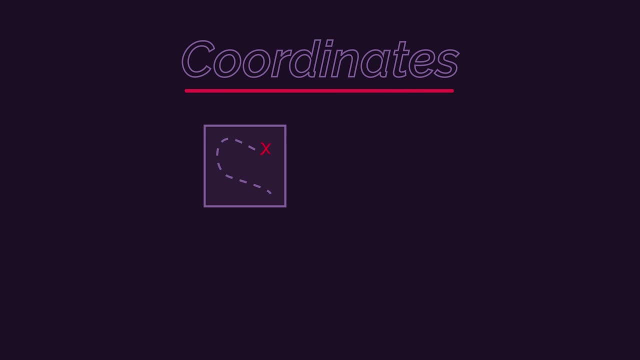 to check. Did you think it was hip? So it's negative. four in this direction and six squares up. Coordinates are really useful for maps, for GPS systems, for computer games, for pixels on screens, And these are known as Cartesian coordinates in honour of the man who developed. 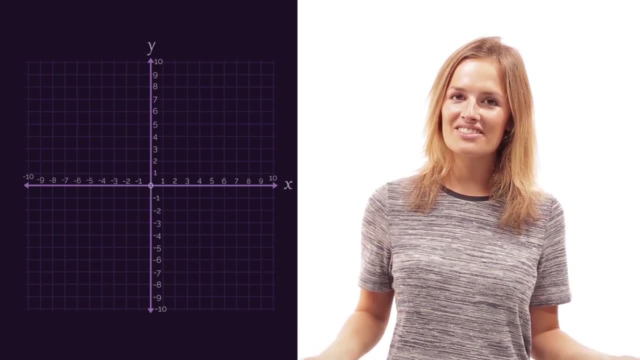 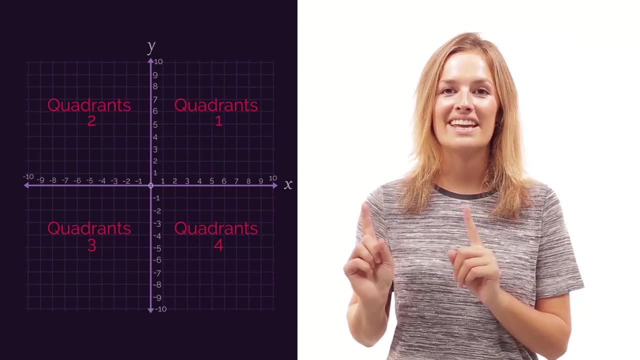 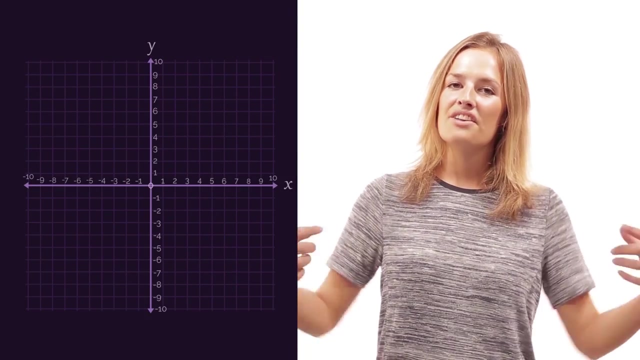 them in the 17th century. Notice how the graph is divided into four sections. These are called quadrants. Notice how they're numbered in an antecedent In an anti-clockwise direction, starting at one and going around to four. 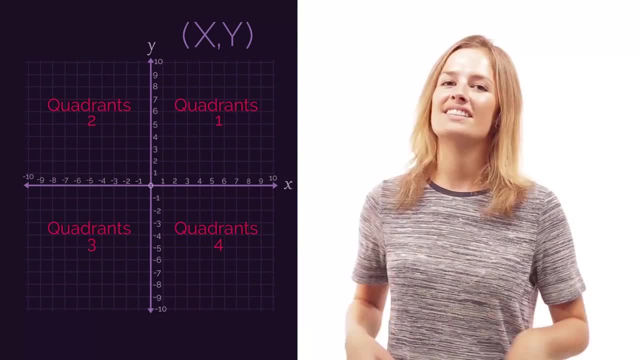 So there we have axes, coordinates and quadrants. In the next video we're going to look at horizontal and vertical lines and two important diagonal lines. 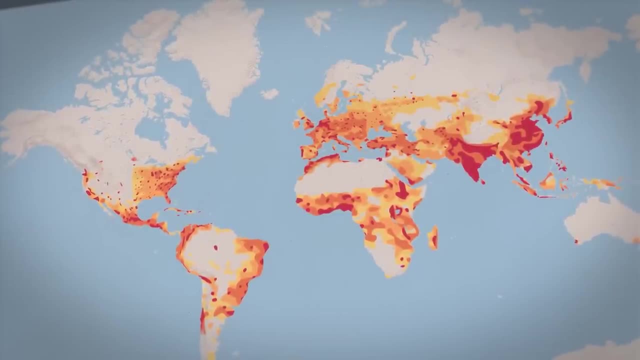 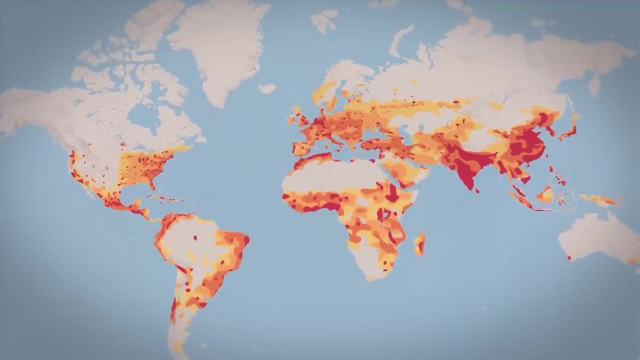 This is a map of where you, me and all the 7.8 billion other humans on the planet currently live. It shows two totally different and separate realities experienced on our planet. The inhabited, populated world made up of cities and settlements of people, where nearly all of us 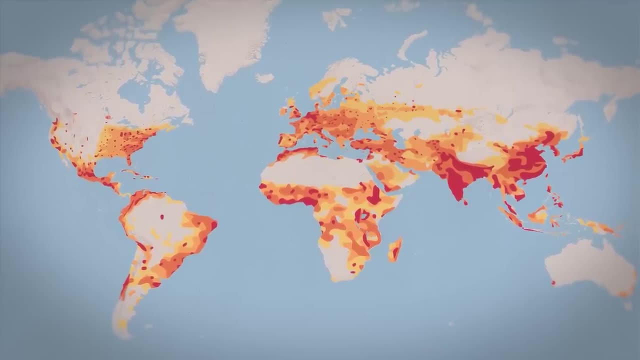 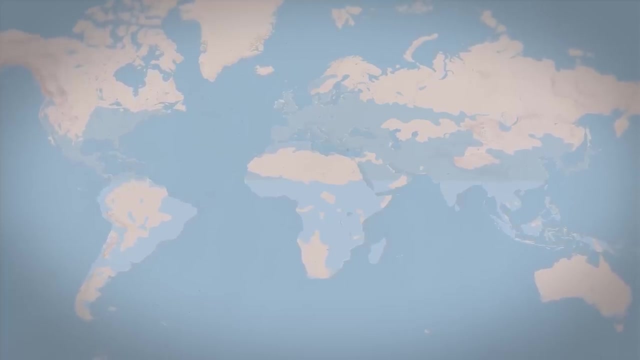 watching this video live in and where nearly everyone you've ever met or heard of exists in. And then there's the rural, under-populated frontiers that are still largely devoid and empty of any of us. This picture tells a million different stories, but the one I want to focus on 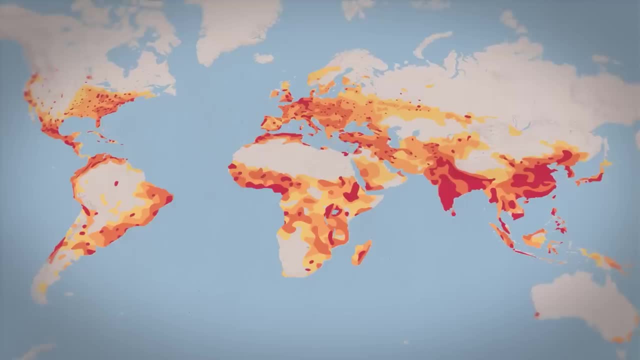 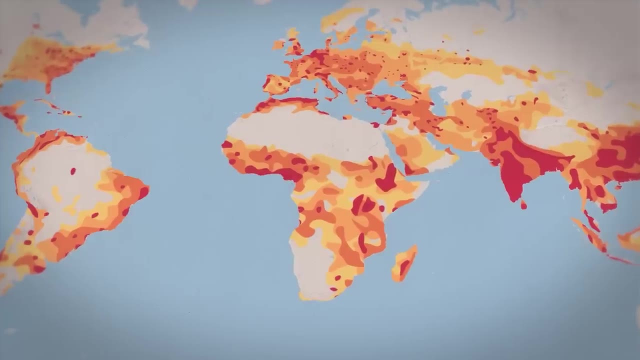 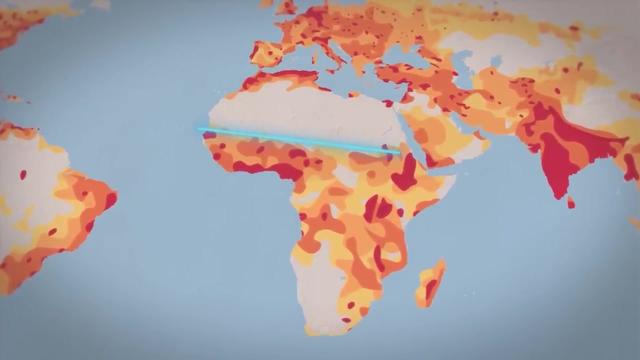 for this video are straight lines. There are only two locations on this map where the settled world and the empty world are nearly perfectly divided by a straight, almost human-looking designed border. The first is here, within the African continent, and it's obvious why it exists. 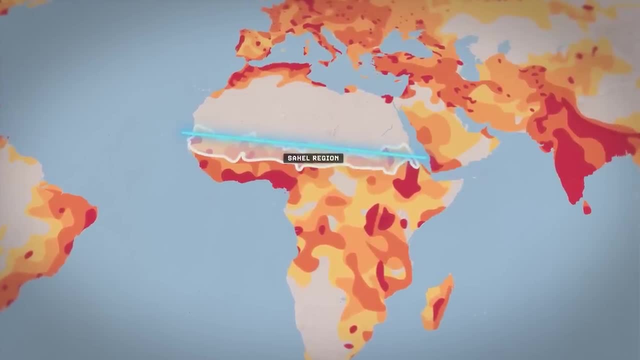 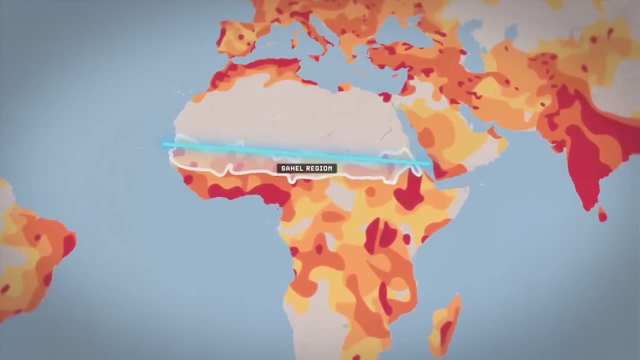 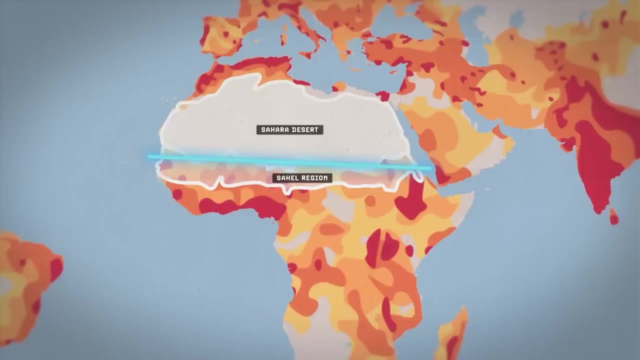 To the south of the line is the African Sahel, a semi-arid belt that wraps across the continent, where rainfall is limited but still actually exists. And to the north of the line is, of course, the Sahara Desert, one of the most hostile environments on the planet to human life. 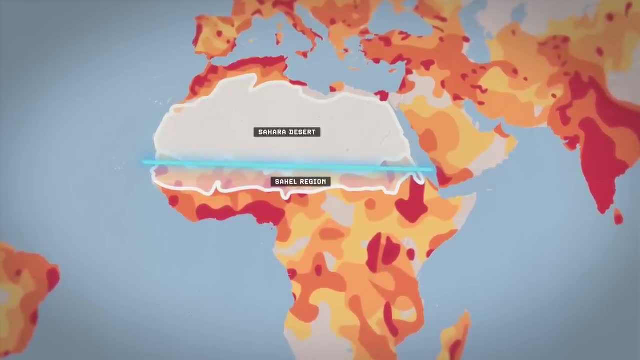 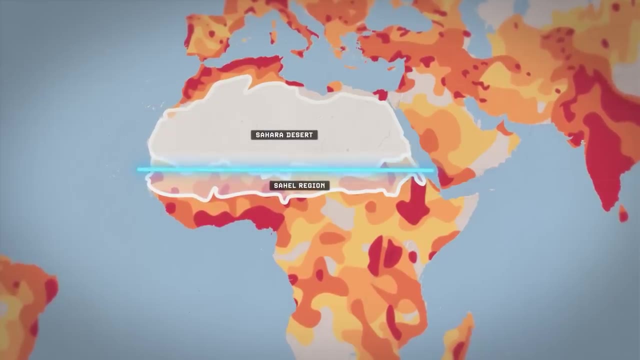 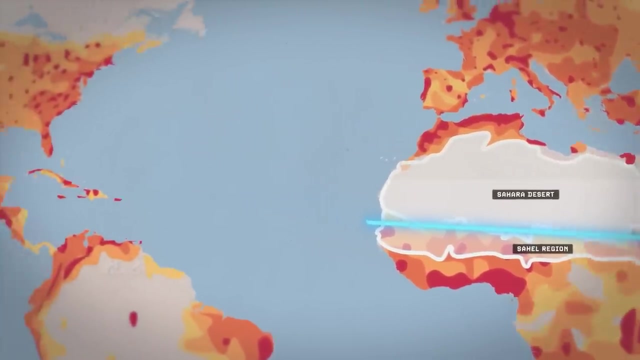 where several years in a row can pass by without a single drop of rainfall and where the average temperature can soar to more than 40 degrees Celsius for months at a time. It's no wonder that nobody lives there, but the other straight-line boundary between the two different worlds of our Earth is significantly stranger.